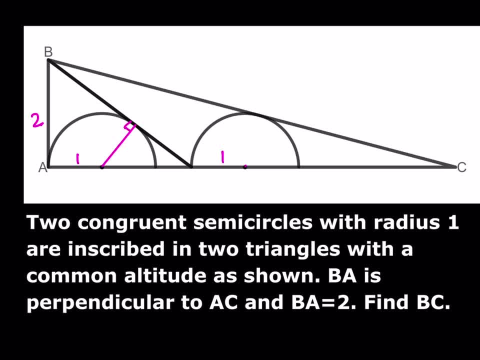 drop a perpendicular that way and then another perpendicular this way. As you know, these are perpendicular lines because the tangent line is always perpendicular to the radius. at that point, Awesome, This is also one, and this is also one. Beautiful. Now, what am I going to do next? I'm 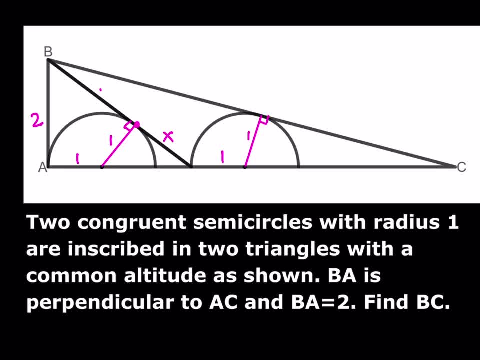 going to call this length here x. As you know, this is also two, because those are two tangents drawn from outside. And let's call this length y here Now from Pythagorean theorem. you know, I don't need to explain in detail. hopefully, right, The hypotenuse is going to be square root of x. 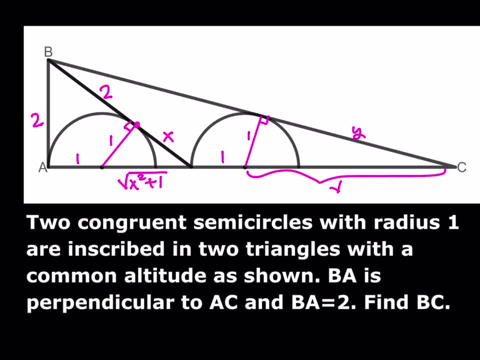 squared plus one, And here it's going to be the square root of y. squared plus one, Nice. So our goal is to find BC, which of course contains y in it. So if you can find those lengths, we can add them up, so on and so forth. Now, what are we going to use here? We're going to use a very nice tool. 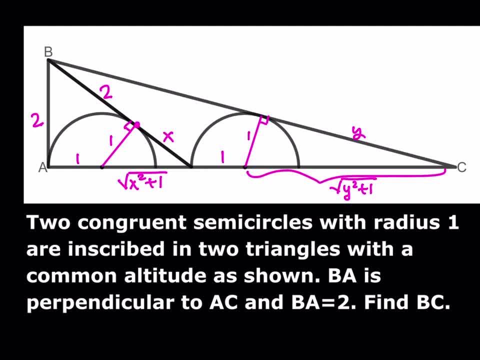 that's used in geometry a lot- in Olympiad problems, in competition problems, in pretty much all types of geometry problems. we use it. It's a really good tool And it's called similarity. Okay, We're going to use similarity here. How Well, if you call this? 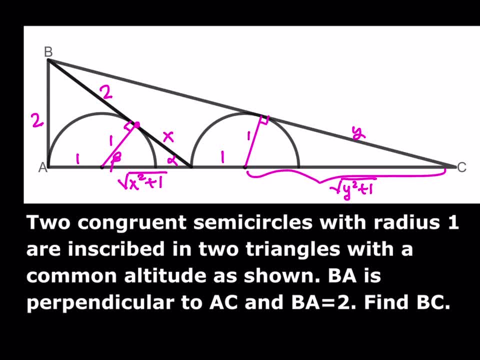 angle alpha, and let's call this one beta. then alpha plus beta is 90 degrees. Therefore, this is also going to be beta. So we have, like an alpha beta 90 triangle, alpha beta 90 triangle, and they are similar. So I'll start with one of the triangles. Let's start with the larger one. 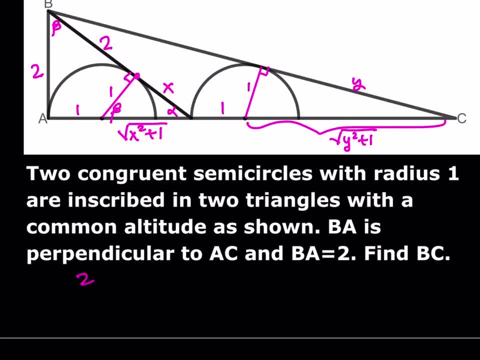 with the alpha. Across from alpha we have the two In the smaller one. across from alpha we have the one. So we kind of have like a two to one. You can tell right And then go back to the big one. What is across from beta In the larger? 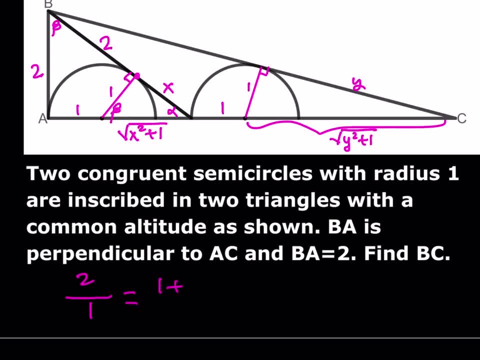 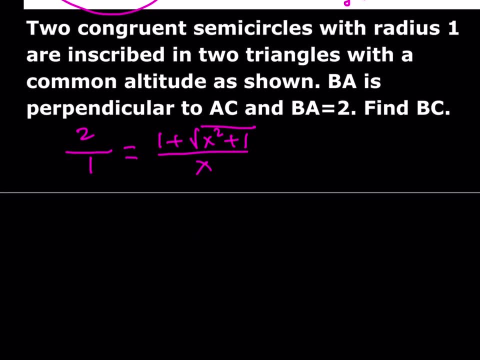 triangle. it's going to be one plus square root of x, squared plus one. I'm talking about this length here, And then in the smaller one across from beta is x. So we're going to put the x in the denominator. So we do have a ratio here, or you can call that a proportion. I guess Let's close. 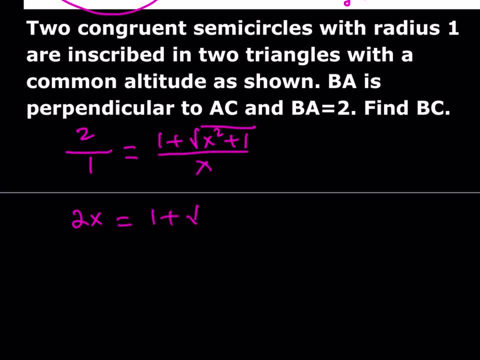 multiply Two, x is equal to one plus the square root of x squared plus one. So we're going to square both sides, But first let's go ahead and isolate the radical. Awesome, Now we're going to square both sides And obviously when you do, you're going to get rid of the radical and you. 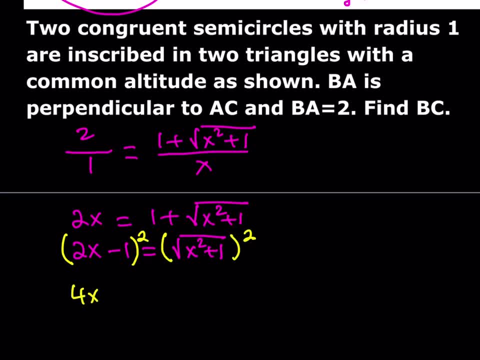 can solve this equation. Awesome. So when you square the left hand side, you're going to get four x squared minus four x plus one. Right hand side is easy: x squared plus one. What's really cool about this is that the one cancels out. Isn't that beautiful? Okay, So you can go ahead and 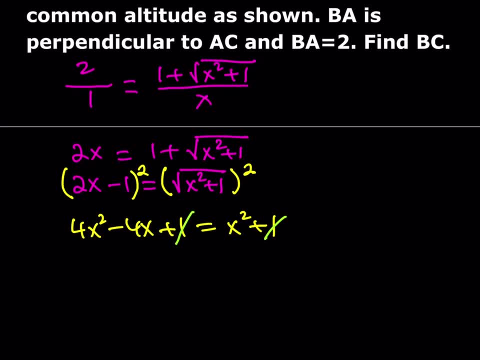 you'll end up with something nicer. Put the x squared on the left hand side, and that should give you three x squared, because you're going to subtract it Beautiful. And then here you can pull out an x, and that should give you three x minus four is equal to zero. Obviously, x can't be zero. 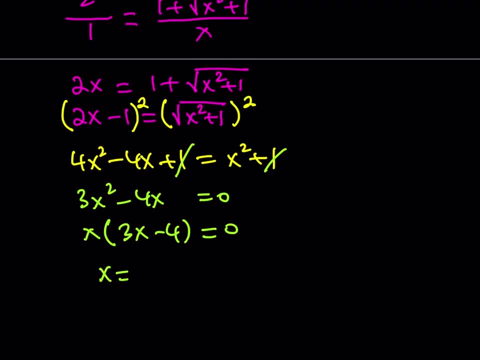 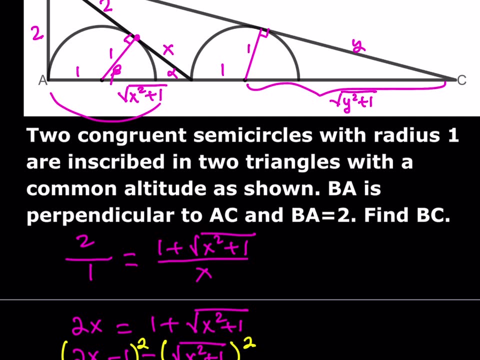 You don't want that right. So three x minus four is equal to zero, which means x is equal to four thirds. Beautiful. Now we found x, We're going to find y. Okay, How can we find y? Hopefully, in. 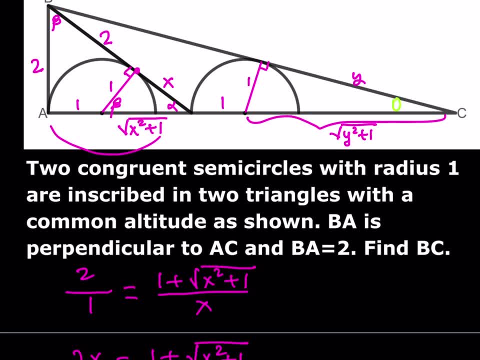 a similar way. right, Can we use similarity? Let's go ahead and find y. Okay, So we're going to call this angle theta, And then in the big one, we also have the theta. Okay, Now, what am I going? 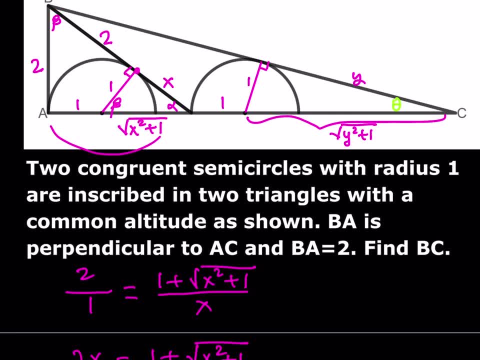 to do. And this is going to be nine to minus theta, right, Okay Cool. And this is going to be nine to minus theta as well. So you see, this triangle is basically similar to the larger one, The largest triangle here. Make sense, Okay, Cool, Because this is a 90 degree angle- Awesome, So we can. 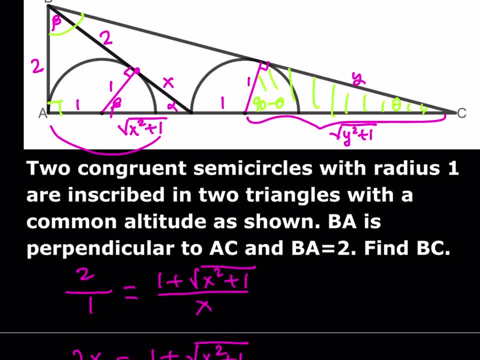 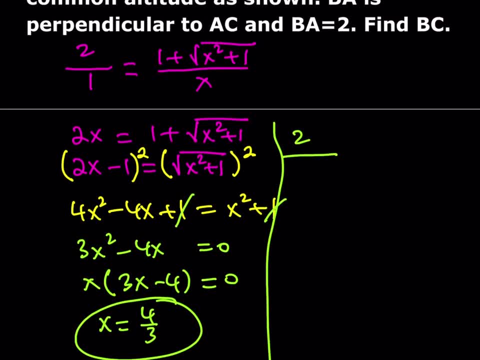 use similarity. The largest one has two across from theta, So let's go ahead and write the two here, Maybe use this area So we're going to be closer And then so theta is two In the smaller one, theta is one, So again we have the. 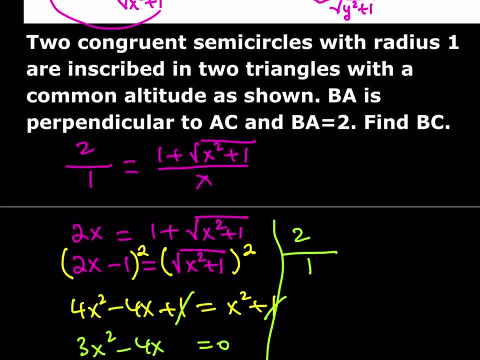 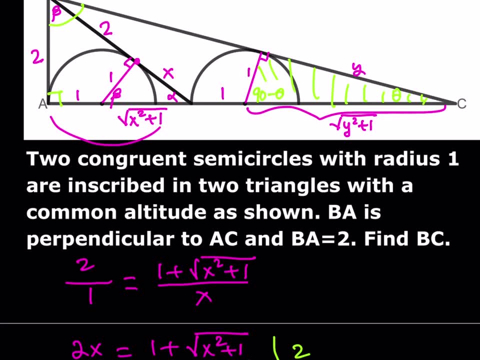 two to one ratio, but this time we're comparing different triangles, obviously, right, Okay, Cool. And in the larger one, what is across from 90 minus theta? That will be the whole thing here: ac. What is ac? Well, ac is equal to one plus the square root of x squared. 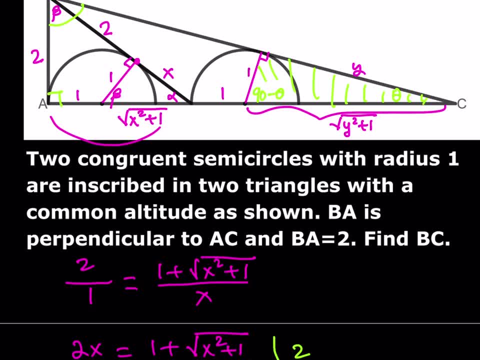 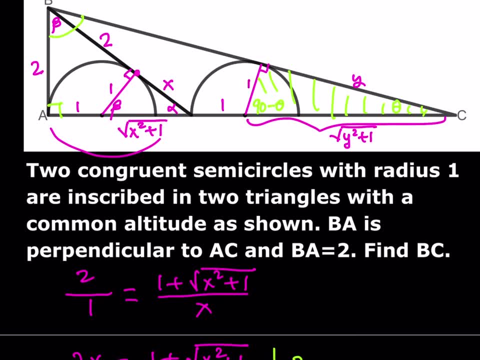 plus one plus one, plus the square root of y squared plus one. But guess what We already know: the value of x. x is equal to four thirds. So the square root of four thirds squared is 16 ninths plus one is equal to 25 ninths. If you take the square root, that's going to be five. 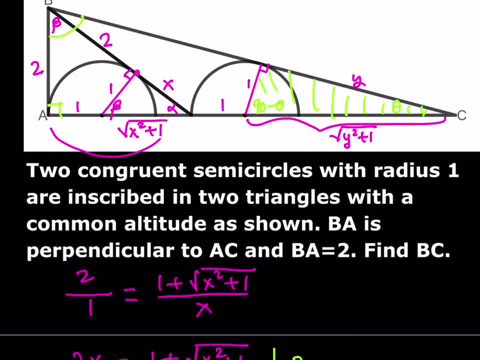 thirds plus one, It's going to be eight thirds plus one is going to be 11 thirds. So this is 11 thirds, this part, right? So you're just going to add the square root of y squared plus one to it. Make sense? Okay, Awesome, Let's check it one more time. Square root of x squared plus one. 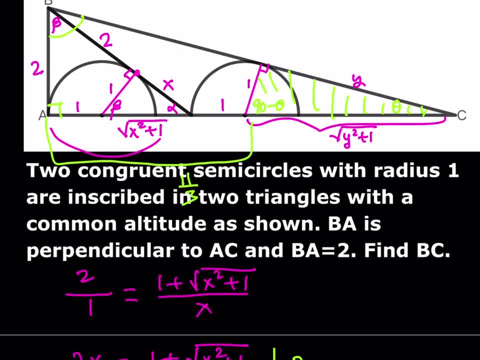 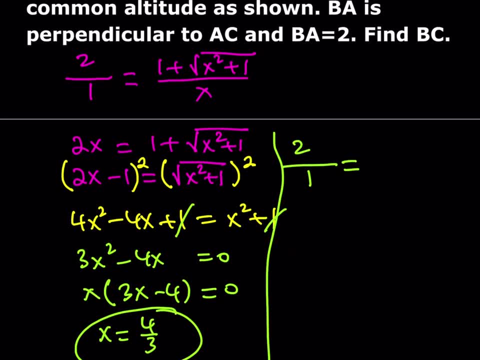 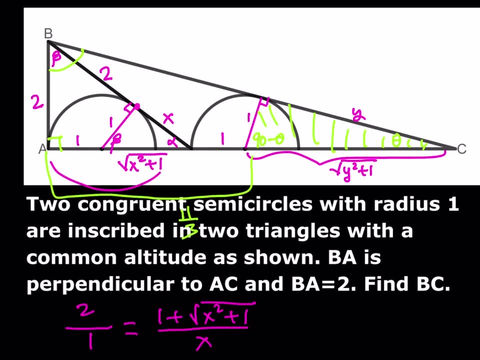 Four third squares is 16 ninths, 25 ninths, five thirds, eight thirds and 11 thirds. Cool, It checks. So we have 11 thirds plus the square root of y squared, plus one for the 90 minus theta, And in the smaller one, the 90 minus theta is y. Okay. 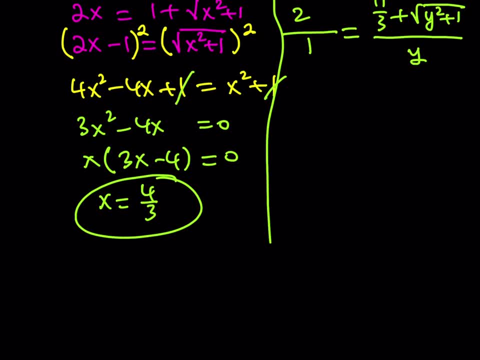 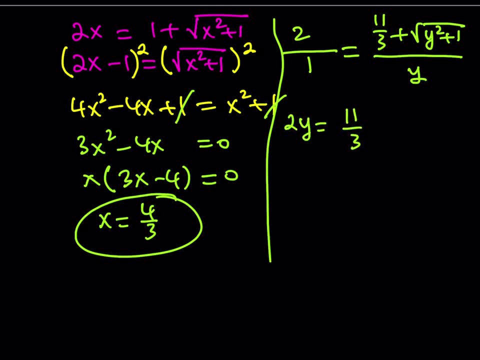 Awesome. So now we have a similar equation for y and we can hopefully solve y from here. Let's go ahead and do the cross multiplication. 2y is equal to 11 thirds plus square root of y, squared plus 1.. Isolate the radical. 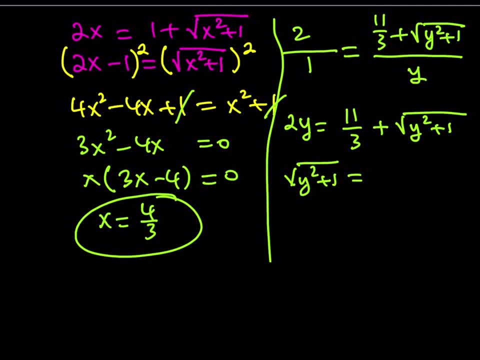 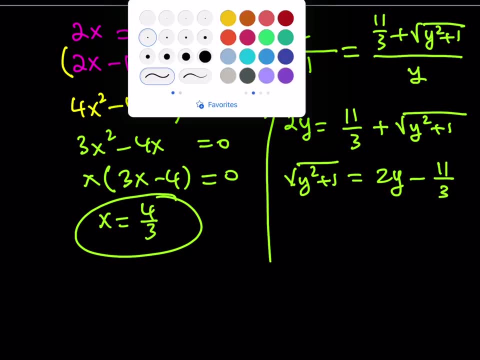 This time I'm going to put it on the left-hand side, which kind of looks a little- I don't know, I guess- better, Maybe not, Okay, And now we're going to square both sides. Now what happens when we square both sides? 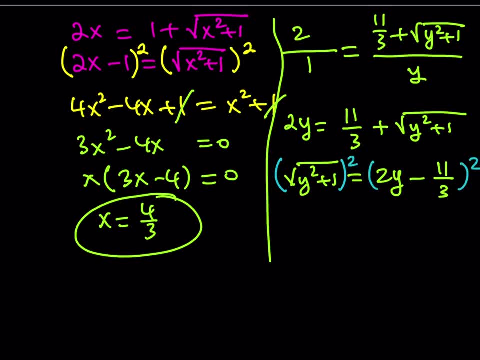 Well, something good happens, because we get rid of the radical, And similarly, we get something nicer: y squared plus 1 is equal to 4y squared minus. Now, when you multiply these two things together, you're going to multiply them. 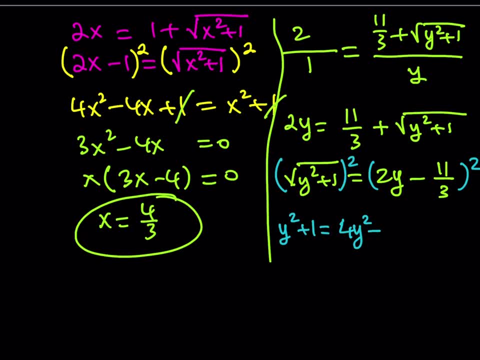 You're going to get 22 over 3y, but you're going to double that right, So it's going to be 44 over 3y, And now you're going to get 121 over 9.. Okay, Awesome. 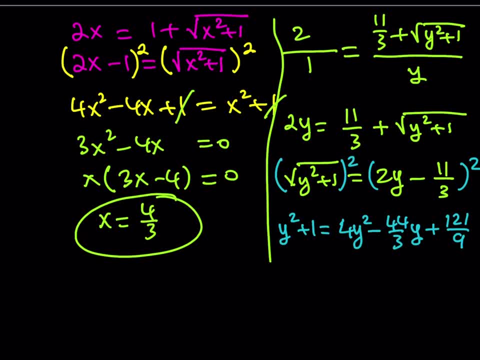 So that's the square of 2y minus 11 thirds. What we can do is we can put everything on the right-hand side and simplify this more. So let's go ahead and do that. here We're going to get 3y squared minus 44 thirds y. 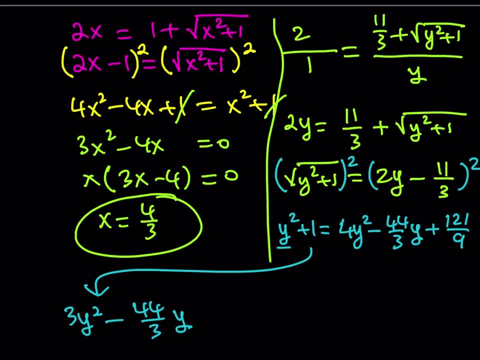 Now I have. okay, I've taken care of this. Now we're going to take care of this: 121 over 9 minus 9 over 9.. What is that going to be? 121 minus 9.. That's going to be 112, right. 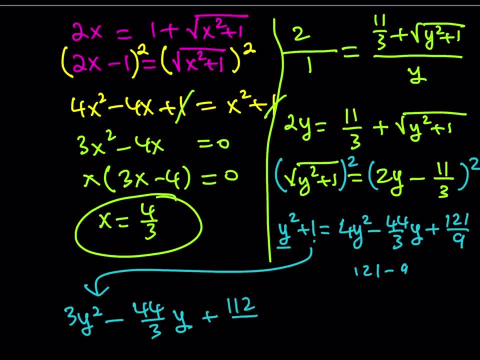 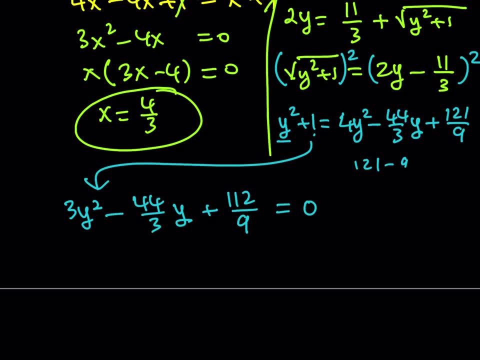 So that's going to be a positive 112 ninths, Great, Okay, And this is equal to 0. Nice, Now, what I can do is obviously that's going to help, right, Multiply everything by 9.. 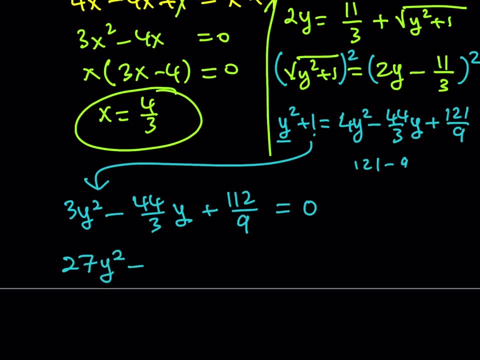 That's going to give me 27.. Y squared minus, I'll get an extra 3 there. 44 times 3 is equal to 132y plus 112 is equal to 0.. Beautiful. Now what am I going to do next? 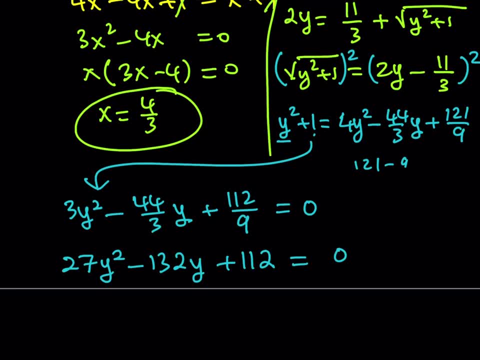 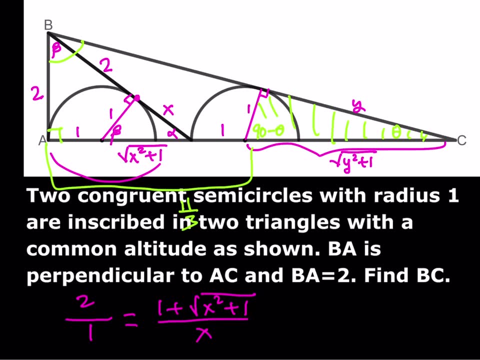 Solve for y, right? Okay, How do you solve for y? Well, to solve for y. and, by the way, after solving for y, we still need to find this length right. How do you find that length? Well, here's the thing. 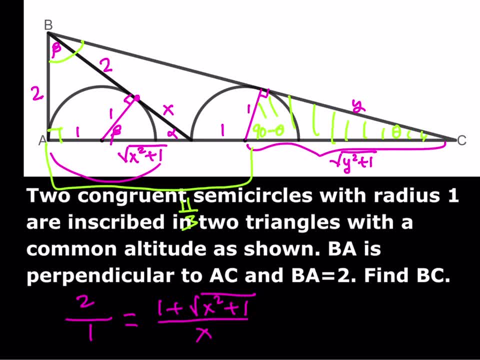 If you know the side lengths right, then you can. basically, once you find the y, you know ac and you can actually use the similarity rule instead of using the Pythagorean theorem. I mean, there are two ways to go about it. 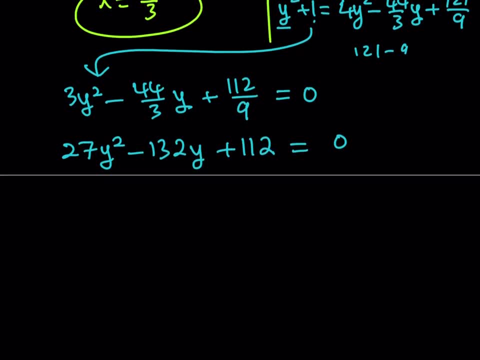 but anyway, let's find y first. Okay, How do you find y from here? Well, let's use the Pythagorean theorem. I mean, what am I talking about? The quadratic formula. Okay, y is equal to negative b plus minus. 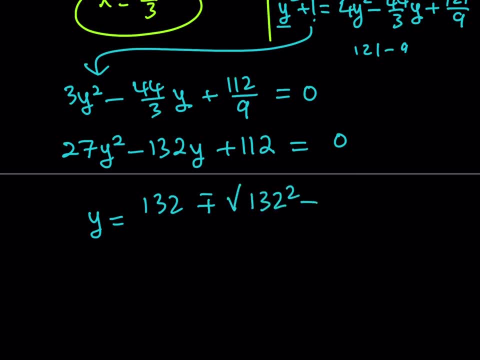 the square root of b squared. Oh man, That's a large number Minus 4ac. Okay, Cool, All over 2 times a, which is 54.. Nice, Okay, So we're going to find the y value from here. 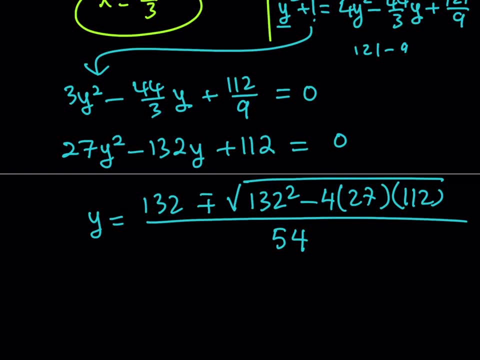 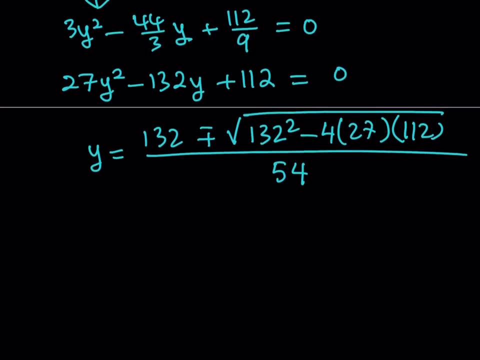 but let's go ahead and simplify this a little bit, because these numbers are too large. Okay, How can we simplify this? Well, think about factoring 132 here. 132 is obviously 2 times 6 to 6, right? 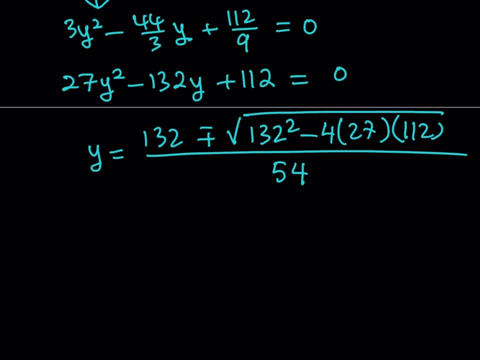 So I can kind of factor it as 2 times. let me do this, Okay: 2 times 6 to 6, and then I could probably write it as 2 times 3 times 11 times 2.. So we can write it as 2 squared. 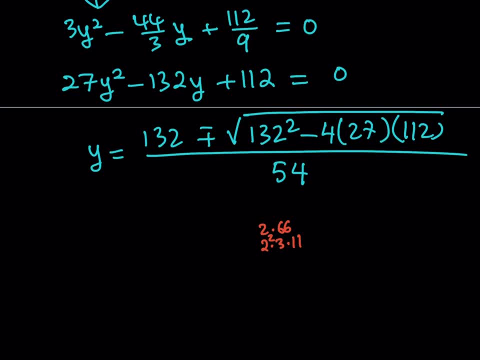 So, in other words, I'm doing prime factorization and then, if I do it for the other piece, 2 squared, 3 cubed and 112 can be written as, let's see, 4 times 28,, right. 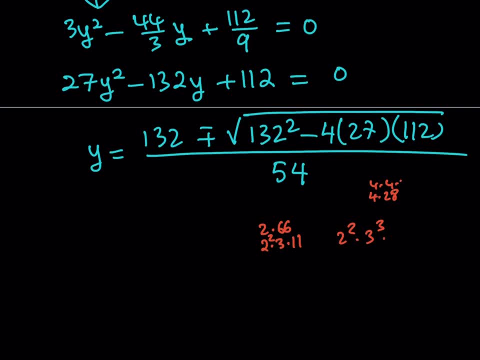 Is that correct? Okay, And then 4 times 4 times 7, which is 2 to the 4th, power times 7.. And this is going to give you basically 2 to the 6,, 3 to the 3rd and 7.. 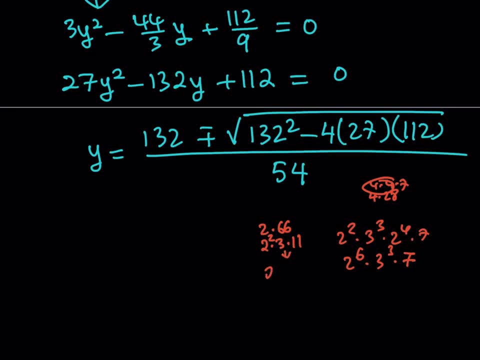 But this guy is squared here. So when you square that, it's going to give you 2 to the 4th, 3 squared and 11 squared. Obviously 11.. Or 7 is not a common factor. 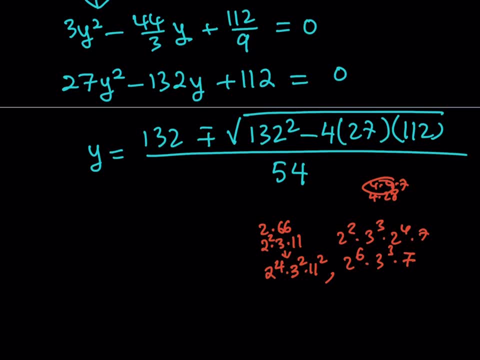 But what I can do is I can basically pull out 2 to the 4th and 3 to the 2nd, which is actually pretty good, because that means we're taking out like a 144, which is nice, right, Okay, cool. 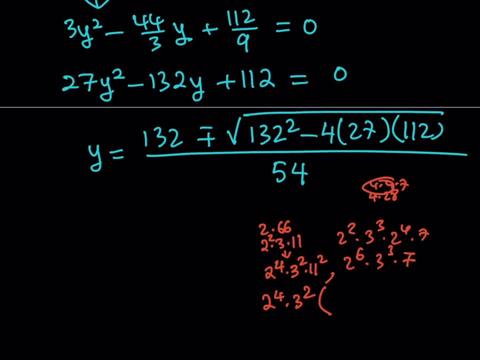 That would be good, And when you factor that out inside, you're going to have: oh, that's actually pretty much everything here, except for the 11 squared. That's kind of nice. Minus, we have a leftover: 2 squared, 3, and 7.. 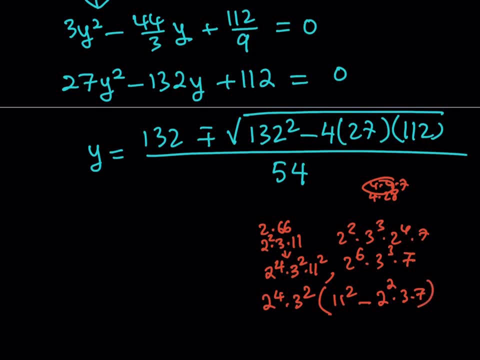 Let's see if this number is left. Let's see if this number is left Less than 11 squared. I'm curious: 2 squared is 4.. 4 times 3 is 12.. 12 times 8 is 84.. 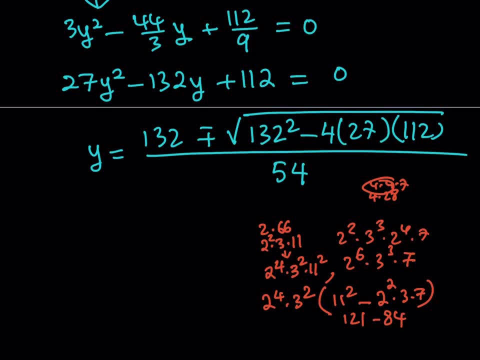 Nice, So it's 181.. What am I talking about? 121 minus 84.. And that should be 37.. Beautiful numbers, right, Okay, awesome. So, basically, to keep a long story short, we can write this as: 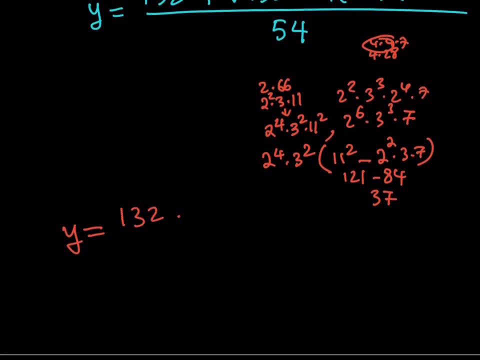 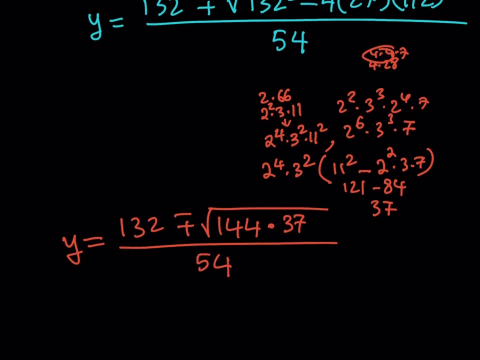 we can write the y as 132 plus minus the square root of 144 times 37.. Isn't that nice? Okay, beautiful, Great simplification. And then we can take this out. If you take out the 144, it's going to be a 12.. 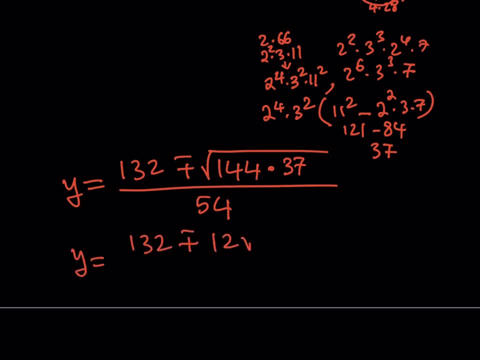 All right, let's see what happens next. That's going to be a 12,, 37 inside the radical and 54.. Okay, common factors: 54 is divisible by 3s and 2s, but not by 4.. 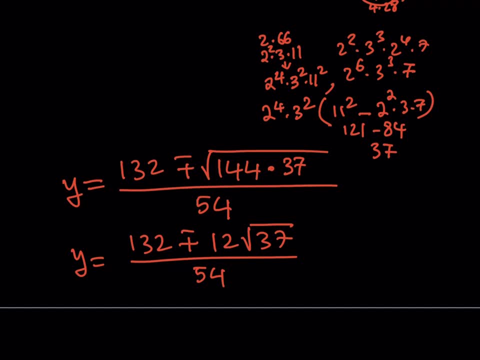 3 is an option, 2 is an option. So that means we can divide by 2.. We can divide by 6.. Beautiful. And if you divide 132 by 6,, what do you get? Well, you get 11,, I think right. 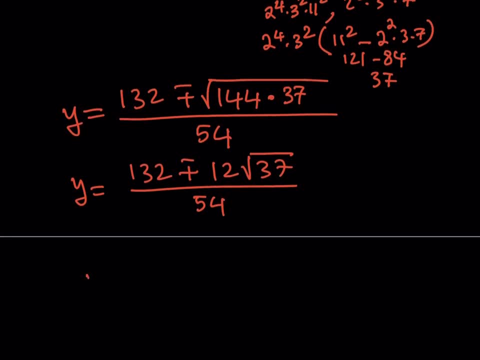 11,. no, I mean 22.. That's what I meant. Okay, divide by 6.. You get 22 plus minus 2 times the square root of 37 over 9.. Now you might be thinking like: which one am I going to use, right? 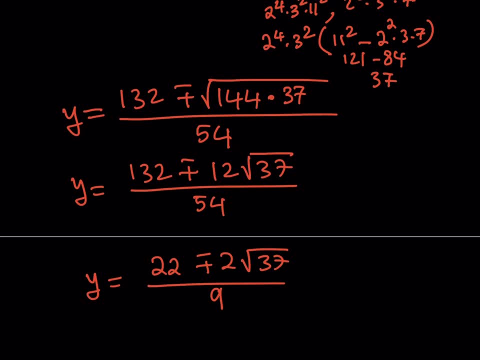 Well, 37, square root of 37 is about 6.. Pretty close 2 times 6 is about 12.. So we're kind of looking at something like this: 12, 22 plus minus 12 over 9.. 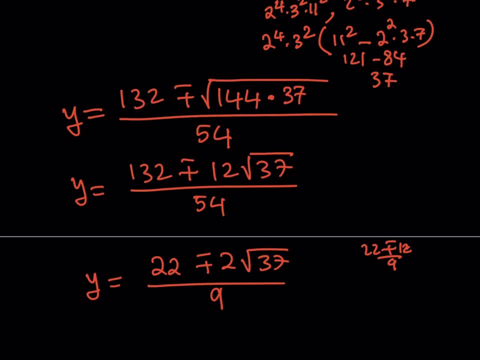 So if you add them up, you get 34 over 9, which is about roughly 5, right, Okay? Nope, that's not 5.. What am I talking about? Okay, sorry, 34 over, it's about, I think, 4-ish, maybe a little less than 4.. 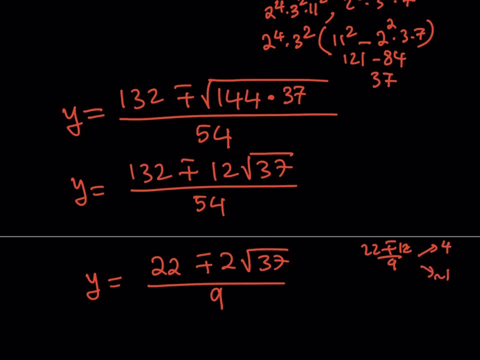 But if you do the 10 over 9, that's going to be close to 1.. Okay, So do you want the y to be close to 1 or close to 4?? Let's take a look at the picture. 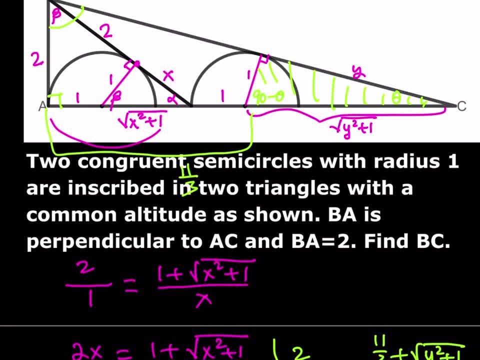 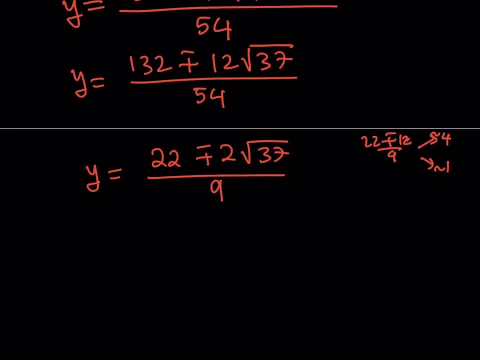 Just eyeball it, you know Well. obviously y is definitely greater than 1.. And so I'm going to go with the positive version. that looks more reasonable And obviously algebraically you can prove that A the only one that works is the positive one. 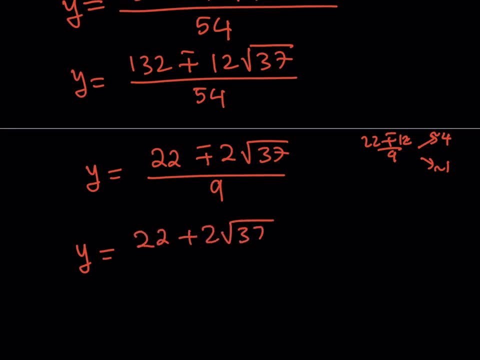 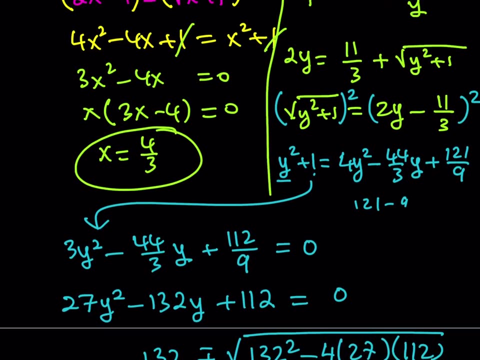 But, anyways, we're just going to keep it simple here. Okay, cool, So this is the y value. Nice, I got the y value. I got the x value. What am I going to do next? Okay, let me tell you what we're going to do next. 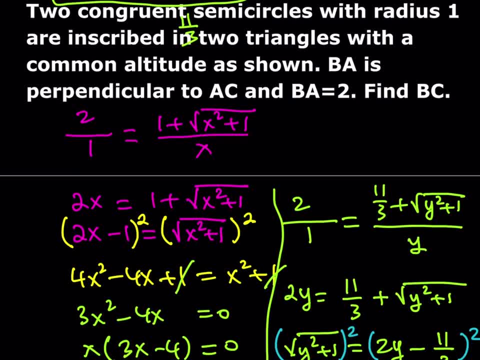 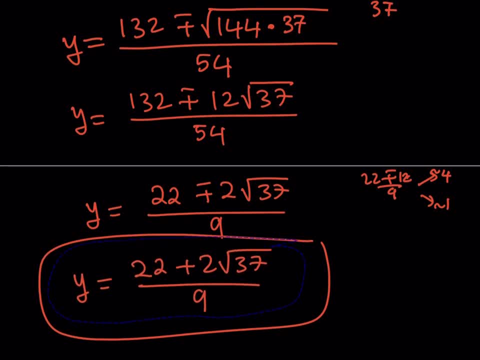 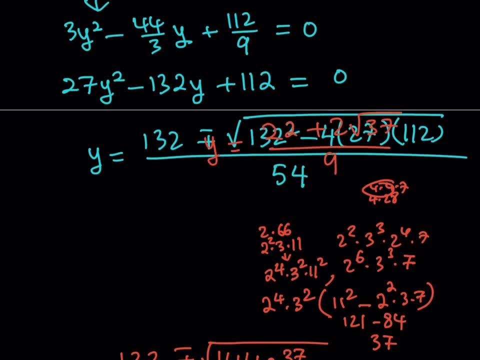 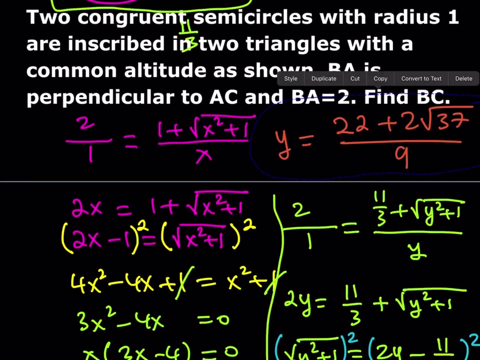 We're going to use these two of these values here. Let me go ahead and do something here. Let me take this little piece here and then move it up. Here we go. I just want to. you know, I just want to put this up here so that I can. you know, it's not easy to scroll down and use it at the same time. 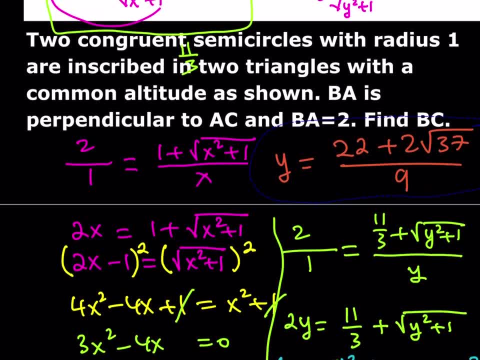 And where's my x value? Oh, x is 4, 3rd. That's easy to do, right? Okay? So let me clean up this area, and then I'm going to go ahead and set up an equation for BC, because our goal is to find BC. 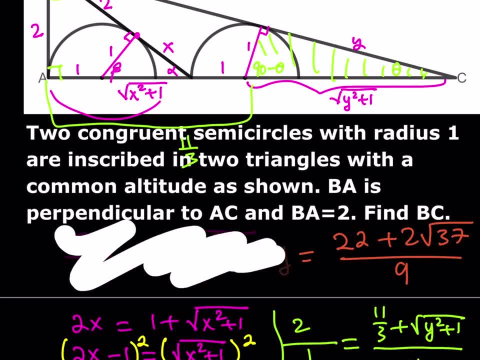 All right, So let me go ahead and clear this area. I don't want to clear the y, So that's my y value And then. so let me clear this area, All right, Cool, Now we know the y value and we know the x value. 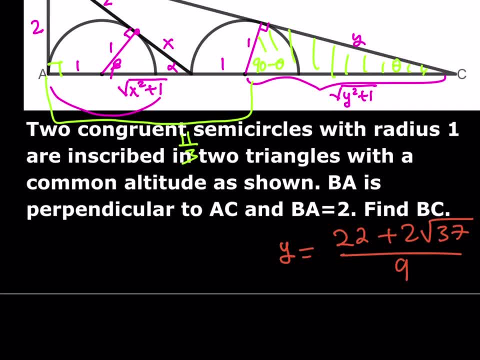 x is equal to 4- 3rd. right Okay, cool, x is 4- 3rd. x is equal to 4: 3rd. Nice Okay, Now what am I going to do to find the value of BC? 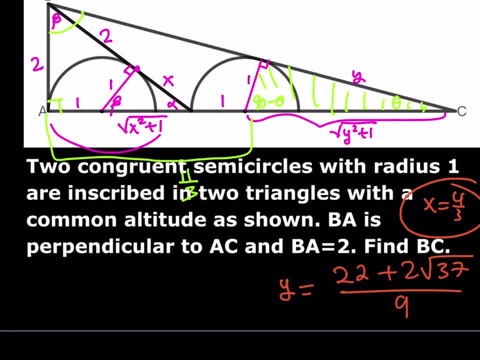 Okay, here's what we're going to do. We do know the value of. well, actually, you can keep it simple. Okay, You want to do it that way? Fine, We can use the Pythagorean theorem instead of similarity. 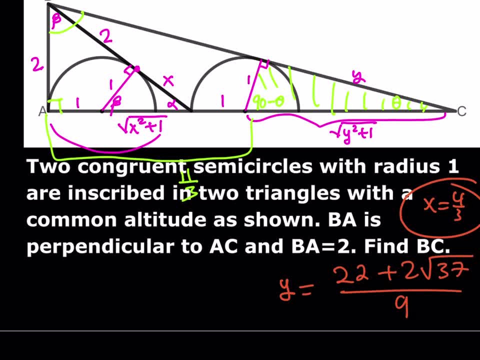 I mean, that's kind of one way to approach it, but I think you will find this probably more helpful. I'm thinking: oh, it doesn't really matter, No big deal. Okay, fine, We're going to find AC and we know AB, and then we're just going to use Pythagorean theorem. 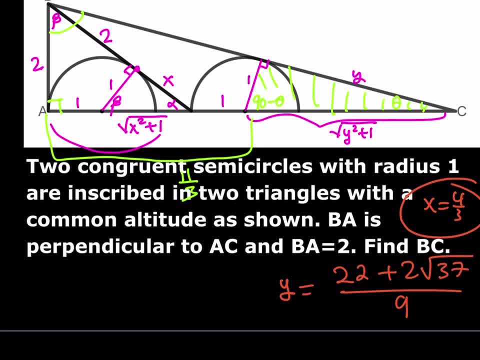 Nice, Okay, cool. So what is AC? AC is equal. to remember, we calculated that already: 11 over 3, right, 11 over 3, plus the square root of y squared plus 1.. Okay, what is that going to be? 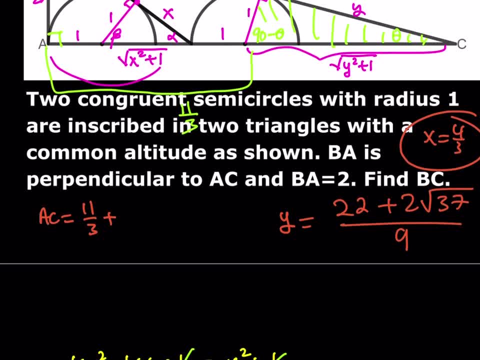 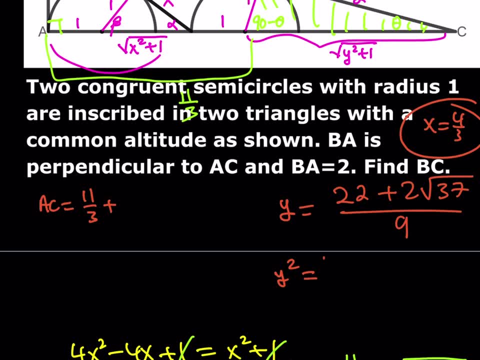 Well, I can just go ahead and square the y, right? If you square y, you're going to get 22 squared. I think that is 484, right, Yep, 484.. Plus, if you square the second term 4 times, 37 is going to be 148.. 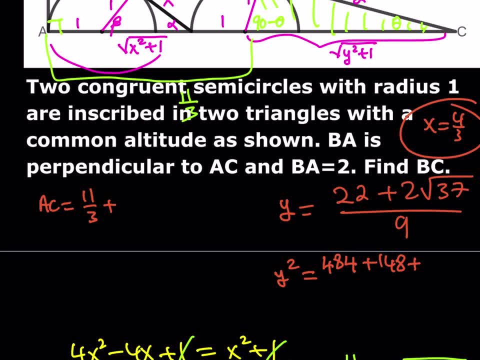 Plus, you're going to multiply and double them, so it's going to be 88 root 37 over 81.. So this is y squared. What you're going to do is you're going to add 1 to this number. okay. 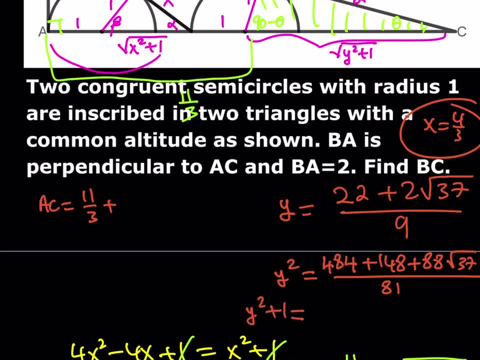 When you add 1, you're basically just adding 81 over 81. So you're going to increase this by 81. So we can add these two numbers and then just add 81 to it, or we can add 81 to this and then add the resulting number. 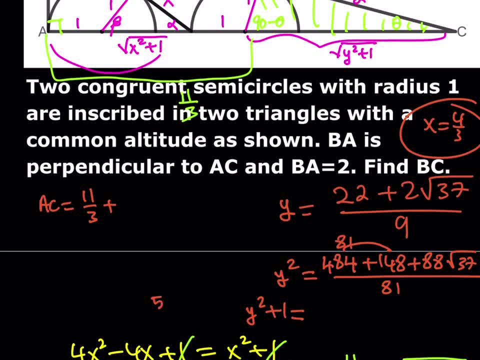 So it doesn't really matter. So that's going to give us 565, and then plus 148.. That should be a 3, a 1, and a 7.. Okay, so that's 713 plus 88, root 37 over 81.. 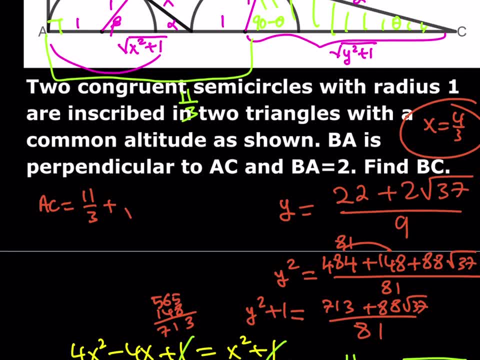 So this is my value And I'm going to square root it and then that's going to give me the answer. all right, So that's going to be 713 plus 88, root 37 over 81,. okay, That's my AC value. 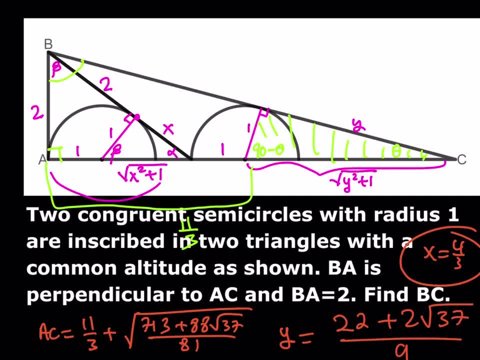 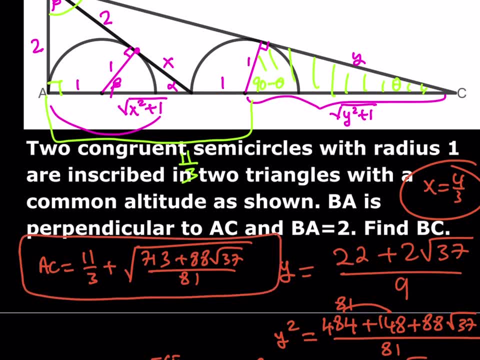 Now, I just got AC, but I got to find BC now, right. But here's one thing to think about: Instead of trying to go through this mess, what I notice here is that you're going to square root this and that's going to be super messy. 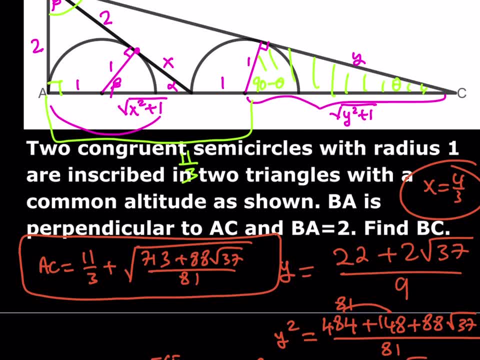 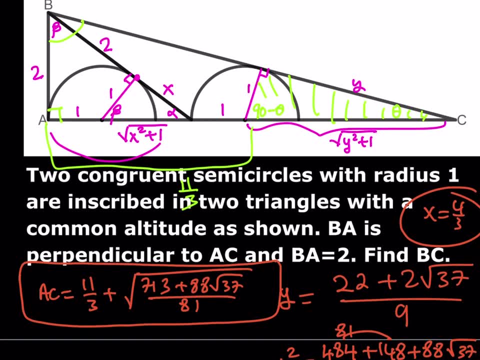 We could just do the following: AC is actually 2 times Y, Why? Because, if you think about the similarity here, we have the 1 to 2 ratio, the smaller one and the larger one, right? So the Y is supposed to be half of AC. 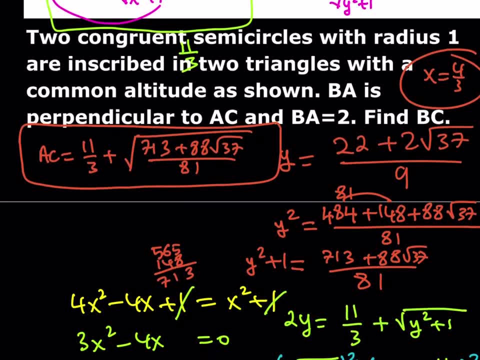 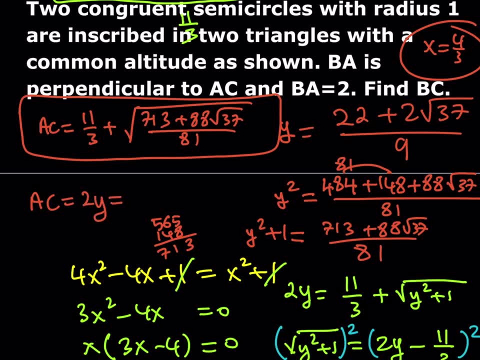 In other words, AC is 2Y. Okay, great, That's actually a really good simplification. So AC is 2Y. This shows us that similarity is a better way to go instead of the Pythagorean theorem. But you will get the same answer no matter what, so it doesn't really matter. 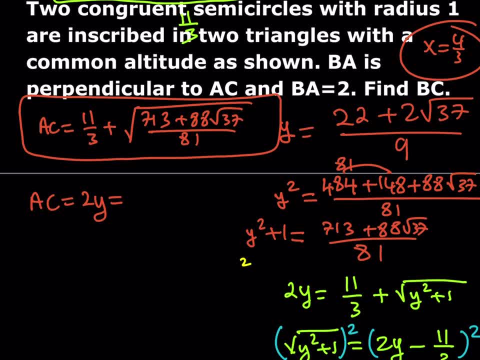 Okay, but this is kind of safer. So 2Y is going to be: we're just going to double it, right? So let's go ahead and double it. It's going to be 44 plus 4 root, 37 over 9.. 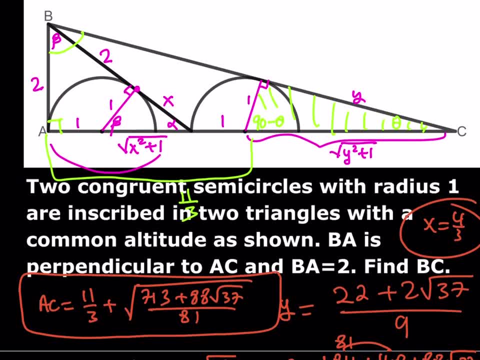 Okay, And again, here you might just use this one. Well, we already calculated this one right, So you might as well say the following too: You can just double this length, right? That's going to be BC. 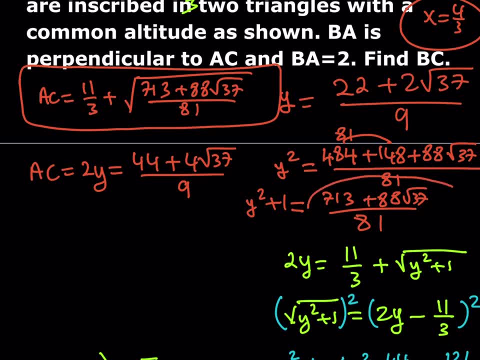 We already found it, didn't we? Okay, so this is my Y squared plus 1. And I can just square root that, right, I can just square root that. And that's going to be 9,, as you know. 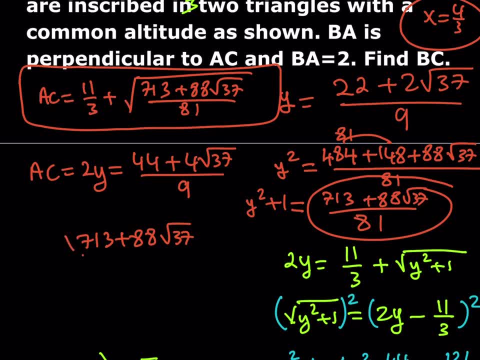 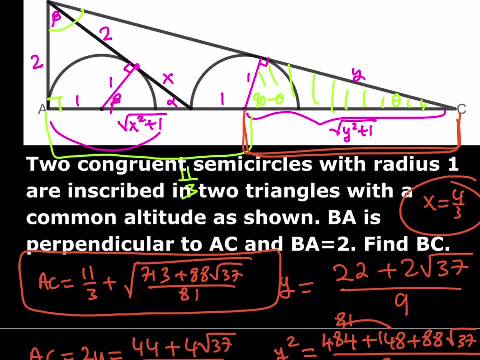 So we might as well just write it like this: Square root of this divided by 9.. Now this is the square root of Y squared plus 1.. So it's this length. here, If you just double it, you're going to get BC. 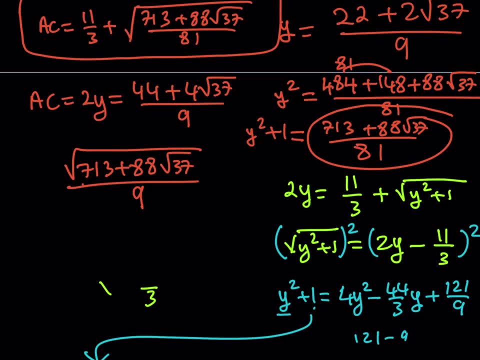 So BC is equal to 2 times this. So case closed- Awesome. This brings us to the end of the video. Thank you for watching. I hope you enjoyed it. I'll see you tomorrow with another video. Until then, be safe and take care.